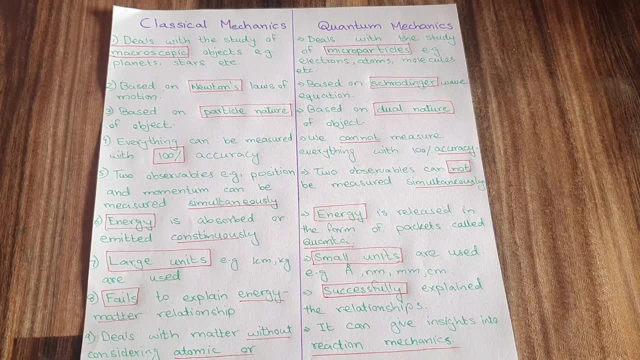 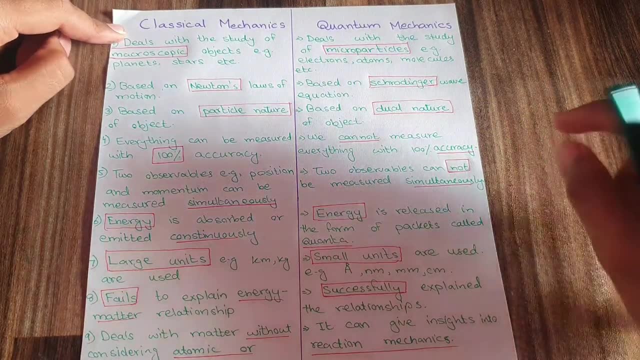 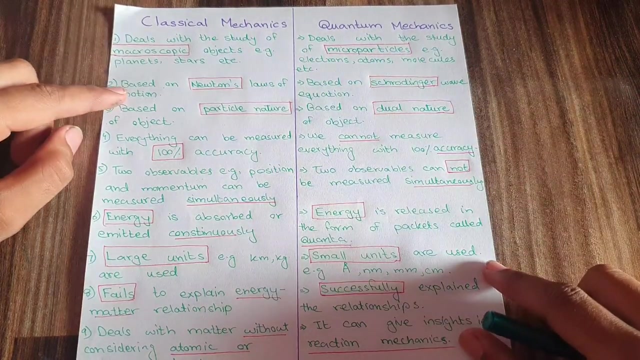 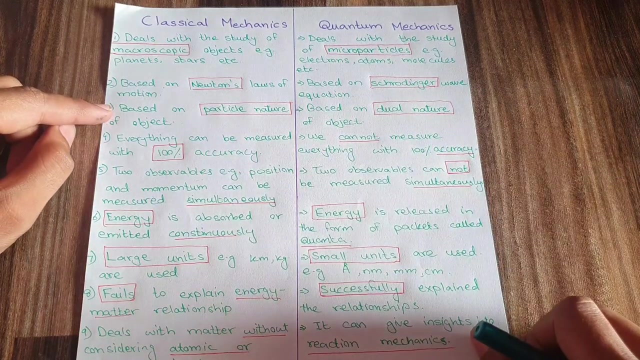 quantum mechanics is used to describe the micro particles, for example the electrons, atoms, molecules. So the classical mechanics applies on macroscopic particles, whereas the quantum mechanics applies on the microscopic particles, the micro particles. And the classical mechanic is based on Newton's laws of motion, whereas the quantum mechanics is based on Schrodinger wave equation. Moving on to the third point, the classical mechanics is based on particle nature of an object. In classical mechanics we only 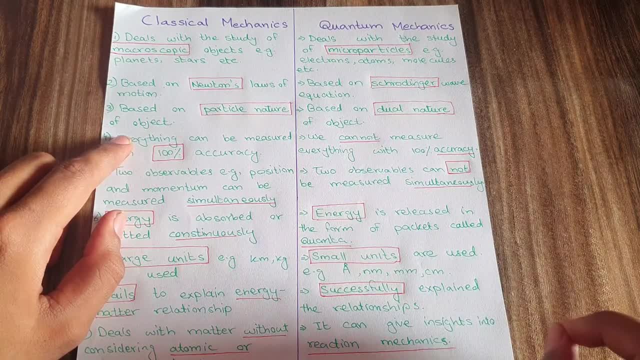 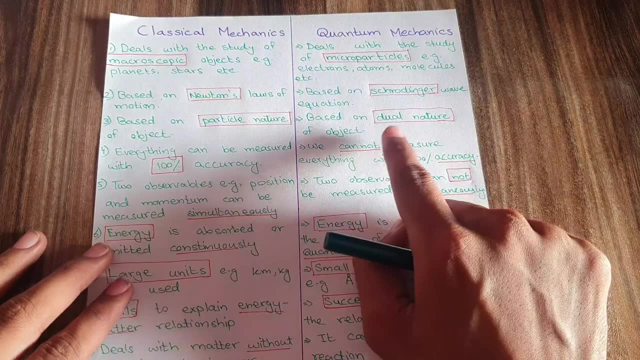 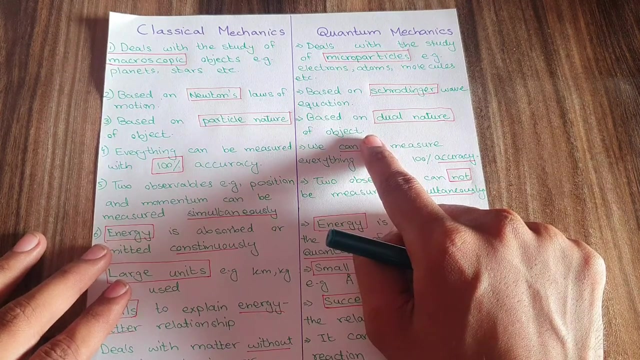 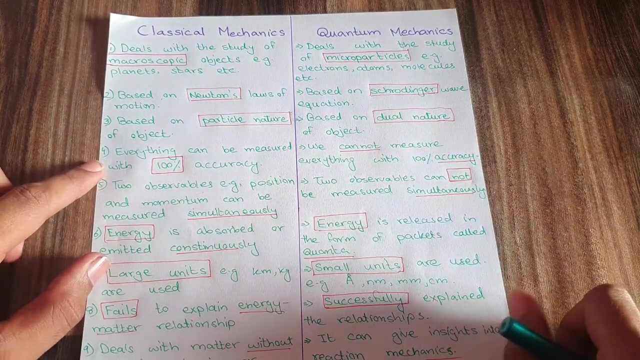 consider the particle nature of object. We only consider the particle nature of object, Whereas if we talk about the quantum mechanics, we have to consider the dual nature of an object, That an object can behave as a wave as well as it can also behave as a particle. So that is the dual nature of an object. And if we move on towards the fourth point, everything can be measured with 100% accuracy In classical mechanics. everything can be measured with 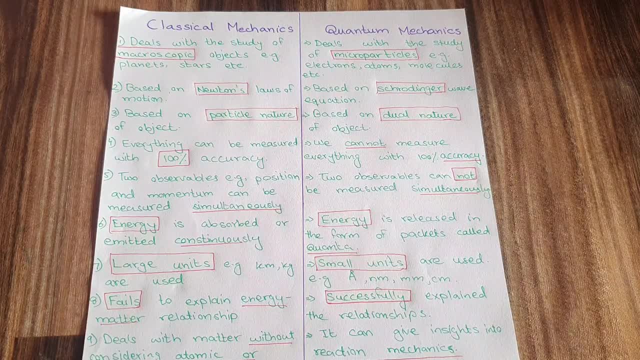 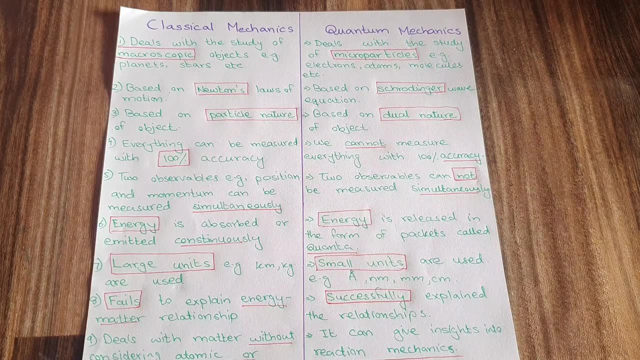 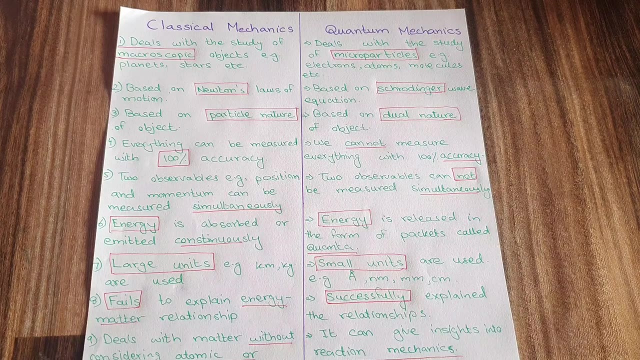 100% accuracy, like if we know the position of a body at one point, we can say we can tell the position of a body at the other point after some time with 100% accuracy. but if we talk about the quantum mechanics, we cannot measure everything with 100% accuracy we have, we are uncertain. 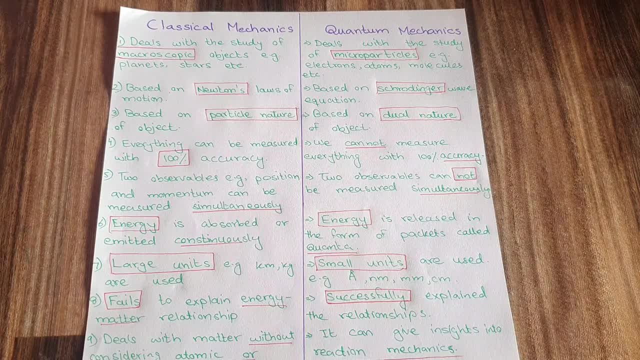 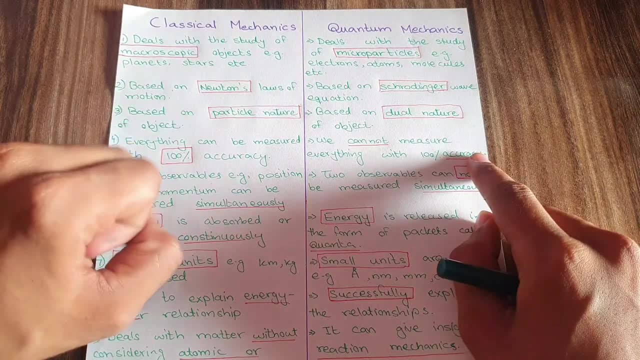 there are probabilities. we can say that, the probability of finding a particle in a place. but we cannot say that the particle is found 100% at a place. for example, if i, if i talk about the electron, i cannot say that electron is found at this place. electron is found at that place, but 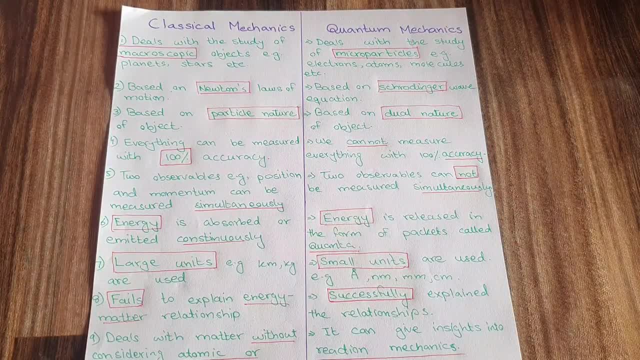 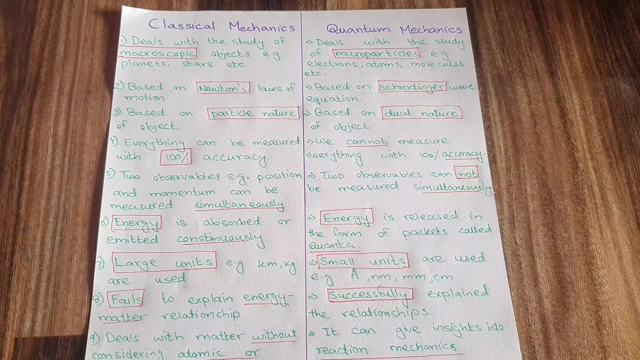 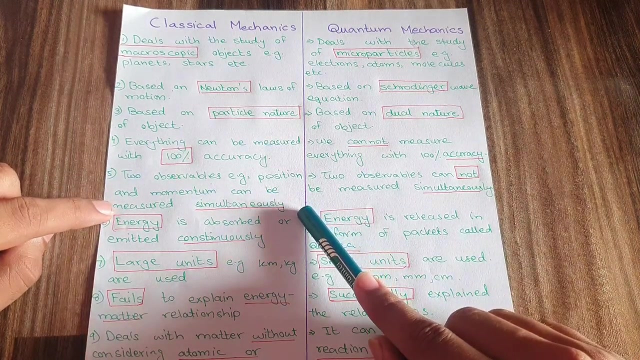 i can say that the probability of finding the electron is maximum at a place. okay, i cannot say that the electron can be found 100% at that place. so the next thing: five, two observations. position and momentum can be measured simultaneously. according to the classical mechanics, position and momentum can be measured simultaneously. 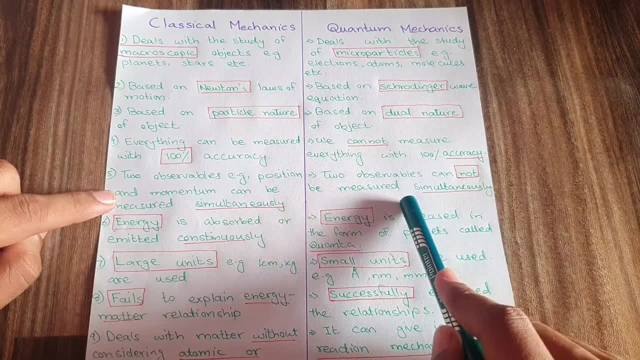 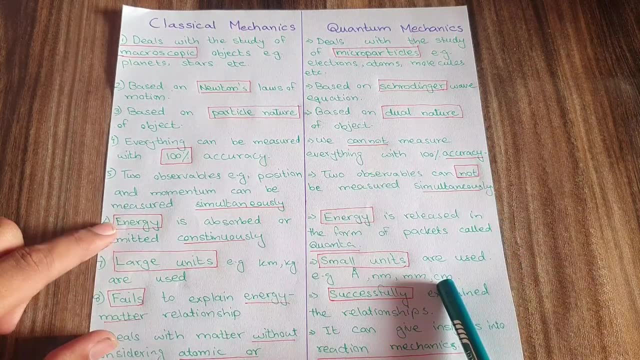 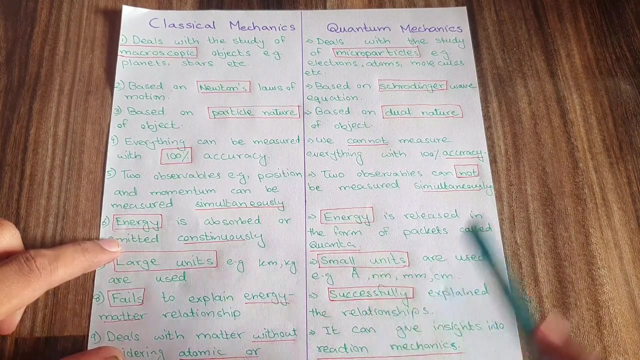 whereas in quantum mechanics the position and momentum cannot be measured simultaneously. that thing we have described in our previous video. moving on towards the point number six, energy is absorbed or emitted continuously. the classical mechanics say that the energy is absorbed and emitted continuously, whereas the quantum mechanics says the energy is released in. 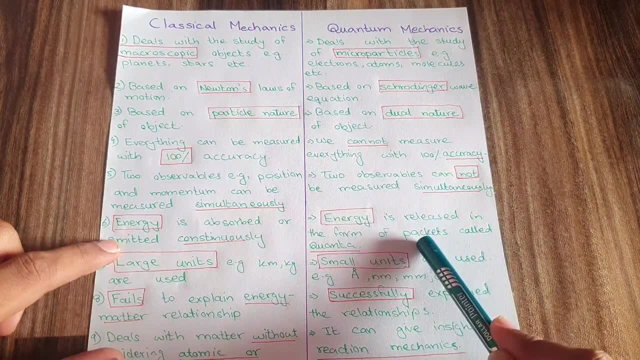 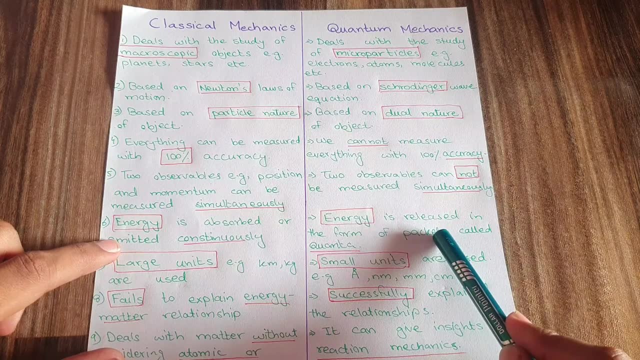 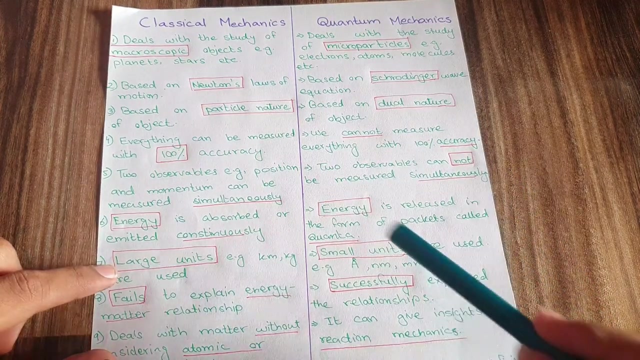 the form of packets called quanta. so the energy is not continuous according to the quantum mechanics. quantum mechanics says that the energy is discontinuous and is released or absorbed in the form of wave packets called quanta. question point number seven: large units. the classical mechanics involves the use of large 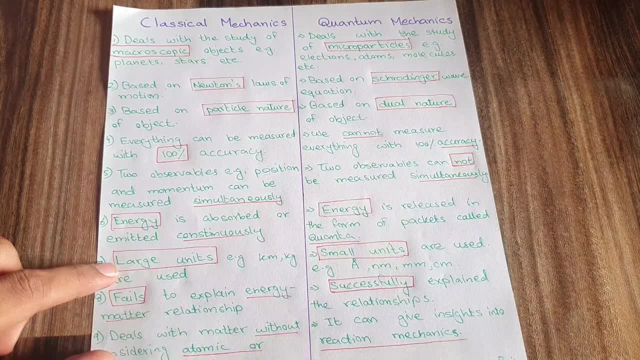 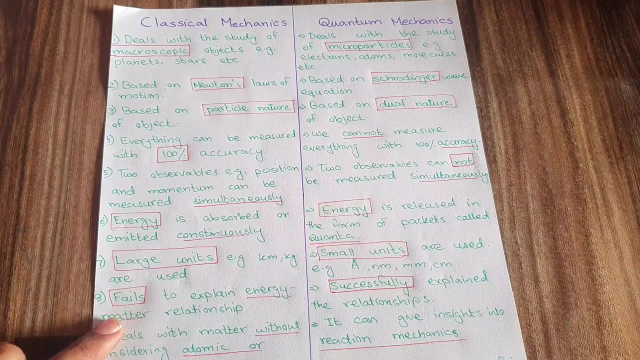 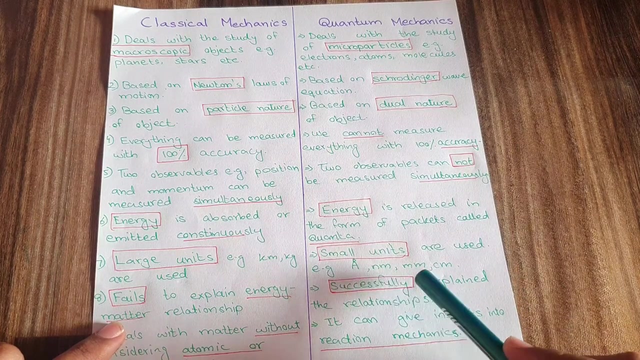 units, since we are dealing with larger objects. so the classical mechanics involved the larger units, for example a kilometer kilogram- are used, whereas the quantum mechanics- quantum mechanics, since it involves the smaller objects, so we can say that the smaller units are used. quantum mechanics, including the angstrom, nanometer, millimeter and centimeter, point number eight. it. 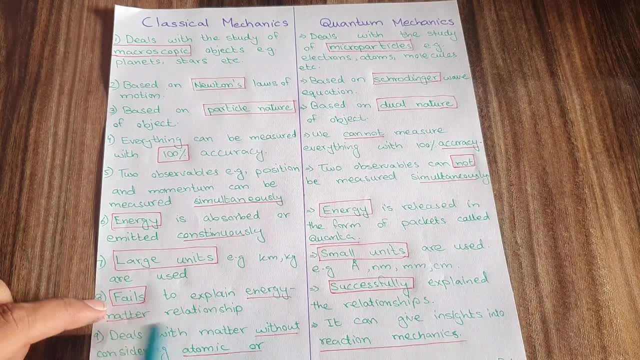 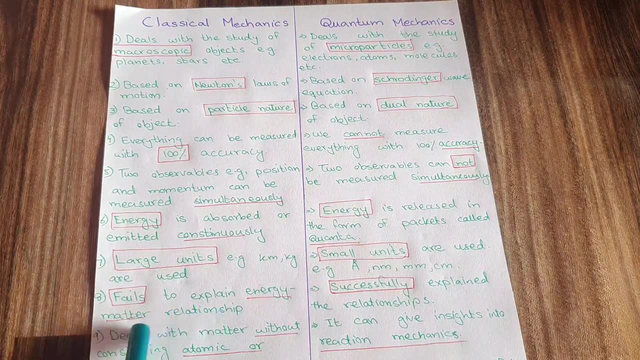 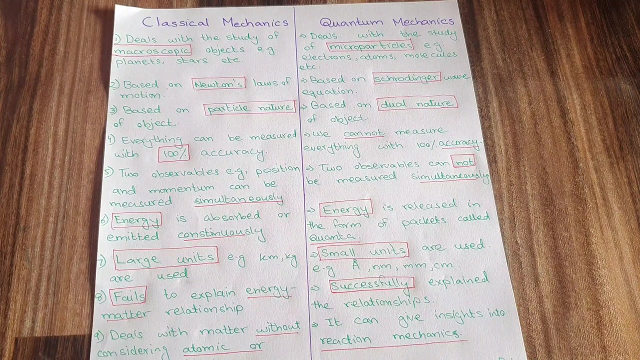 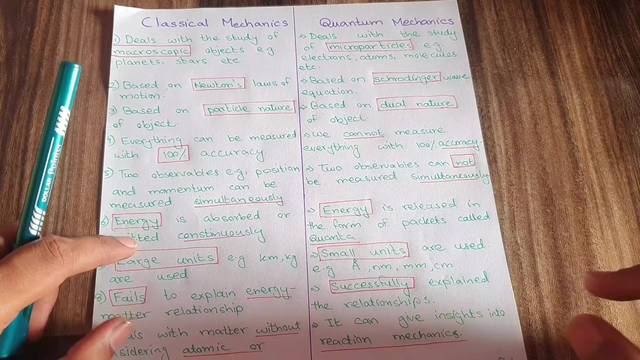 fails to explain the classical mechanic, fails to explain the energy matter relationship. okay, the classical mechanics cannot explain the energy matter relationship that the energy can be converted into. Einstein's said that energy can be converted into matter and similarly the matter can be converted into energy. this thing can only be explained by quantum mechanics and cannot be. 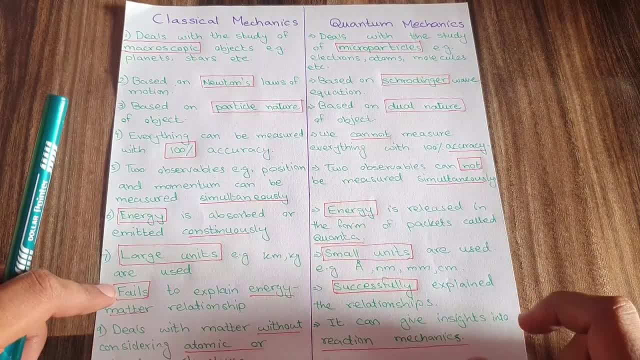 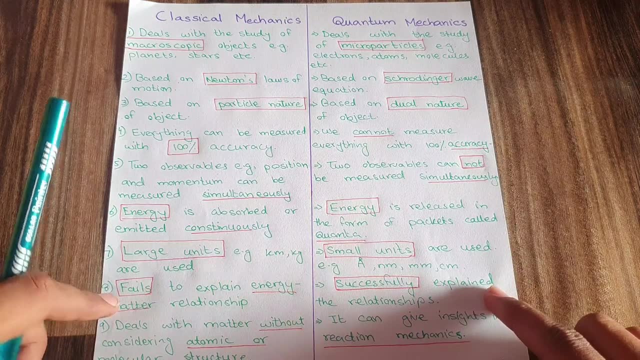 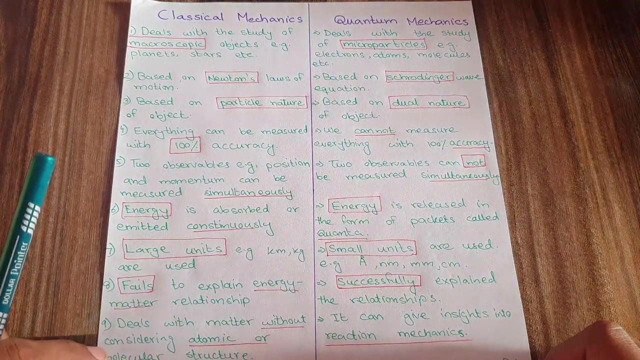 explained by classical mechanics. okay, classical mechanic fails to explain the energy matter relationship, whereas it is successfully explained in quantum mechanics. moving on towards the point number nine, the classical mechanic deals with the matter without considering the atomic or molecular structures. since we have already read that the classical mechanics 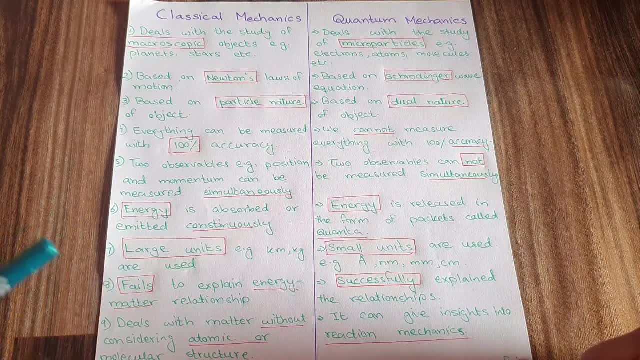 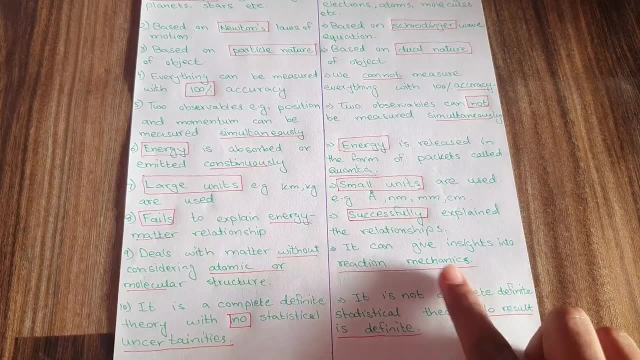 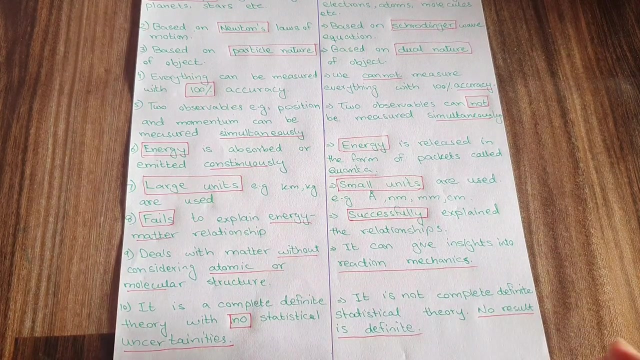 only deals with the larger object objects, so it does not deal with the atomic or molecular structure, whereas if I talk about the quantum mechanics, the quantum mechanics gives insight to the reaction mechanics. it tells us the phenomena occurring at atomic and molecular level. moving on towards the point number ten, it is complete definite theory with no statistical 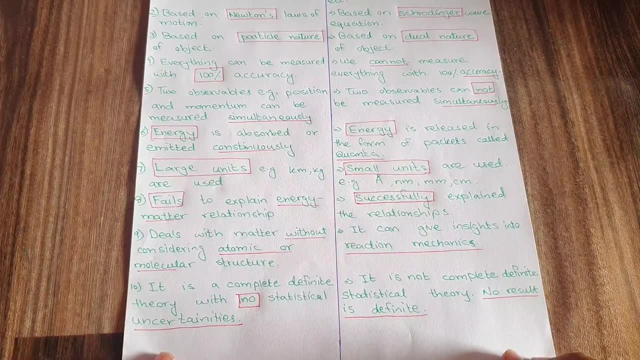 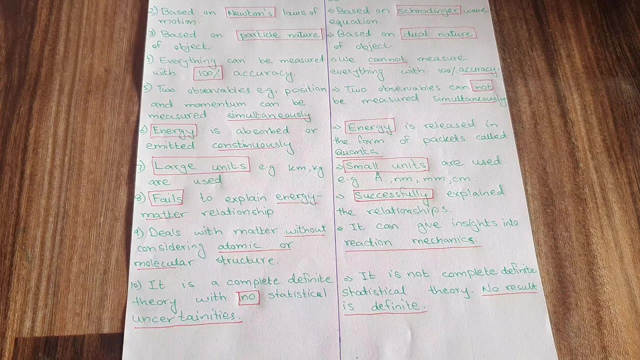 uncertainties. we can say that in in classical mechanics there are no statistical uncertainties. in classical mechanics there are no statistical uncertainties, there are no statistical uncertainties, uncertainties, whereas in quantum mechanics there are only probabilities and there are only uncertainties. we cannot be certain, we cannot be 100 certain about anything in quantum mechanics. 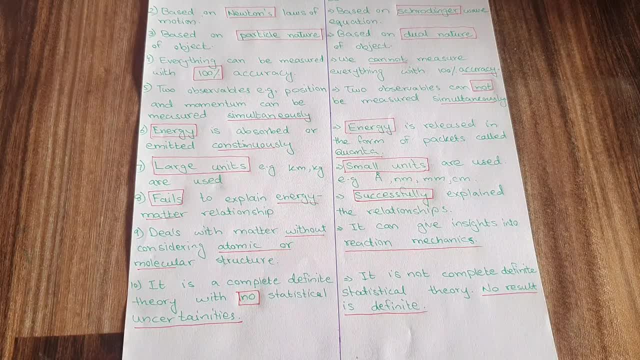 okay, so these are the 10 differences between the classical mechanics and the quantum mechanics. inshallah, moving on. uh, see you in the next video. do not forget to like and subscribe the channel, thank you.